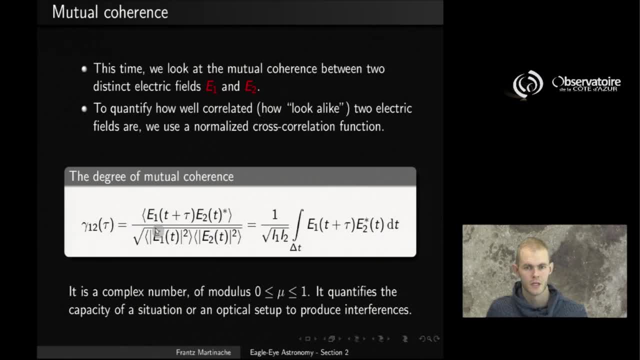 the time-average correlation between E1 and E2 and normalized by the modulus of both E1 and E2.. Now you know that, because we've introduced these things before, that the time-average modulus of E1 and E2 happens to be what we've called the intensity. 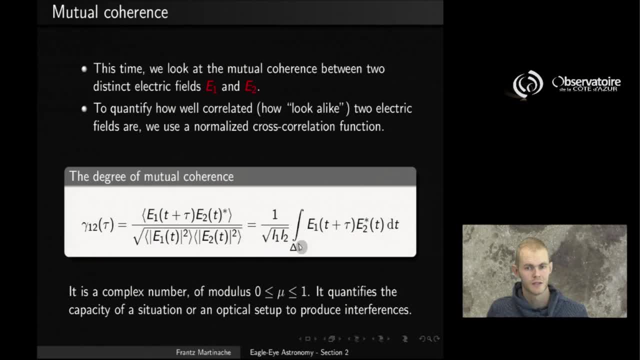 And so that normalization here just greatly simplifies. It's just the square root of the product, of the intensity of those two, And the way we write this time averaging is by integrating over time the cross-product between the two fields. Just like before, it's a complex number. 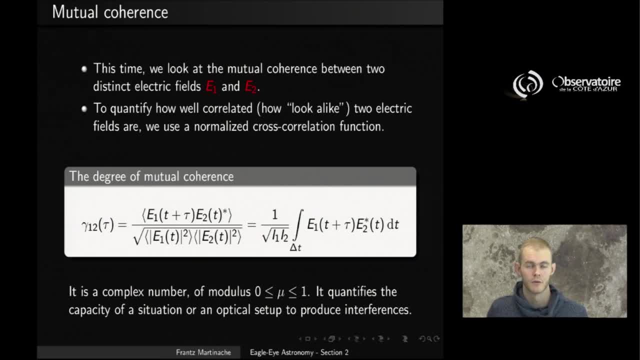 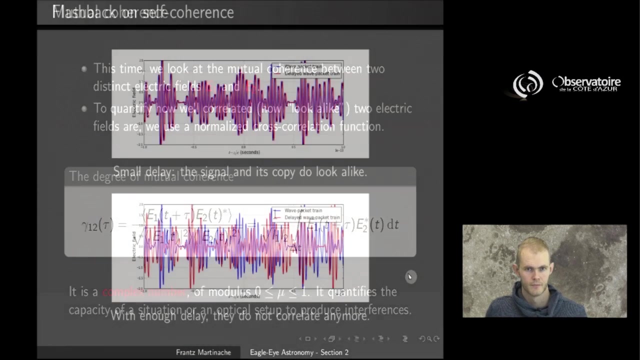 characterized by a modulus whose magnitude is going to be between 0 and 1.. And how close to 1 that modulus is quantifies the capacity, the opacity of a situation or an optical setup to produce the phenomenon of interferences. If we go back to the case of self-coherence, 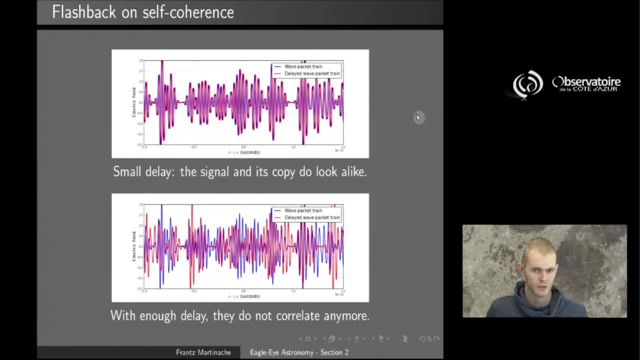 remember that we've said that. well, when two signals are slightly delayed in time, so one signal and its copies are slightly delayed in time, the self-coherence can be quite strong. But with enough delay the two signals look so different from each other. 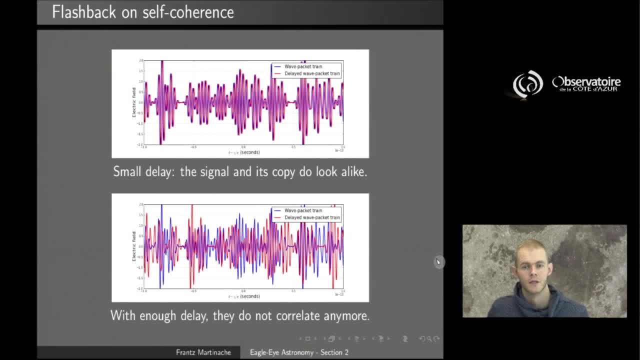 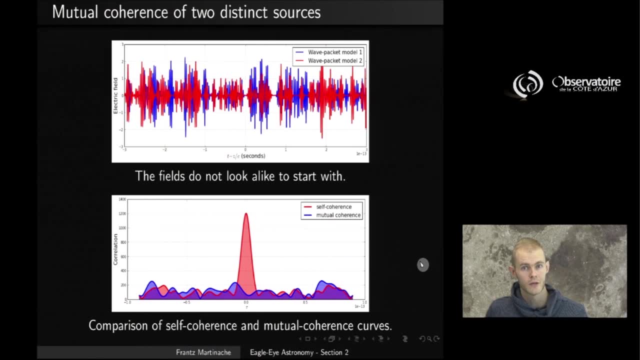 that they are going not to correlate at all. Well, imagine what's going to happen if you go and look at the mutual coherence of two distinct sources, And this is typically like a simulation of what the electric field would look like over a very small time scale of about 10 to the minus 13 seconds. 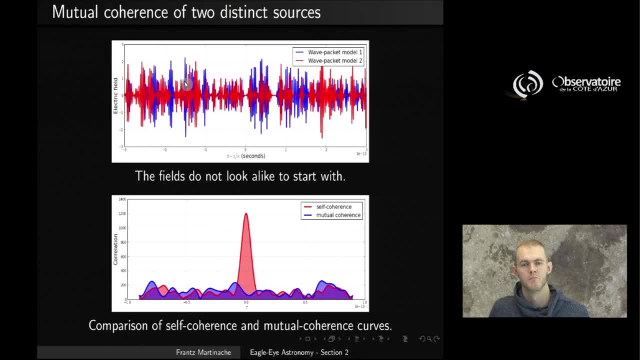 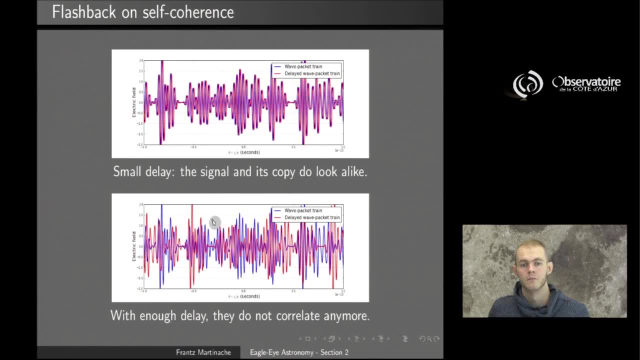 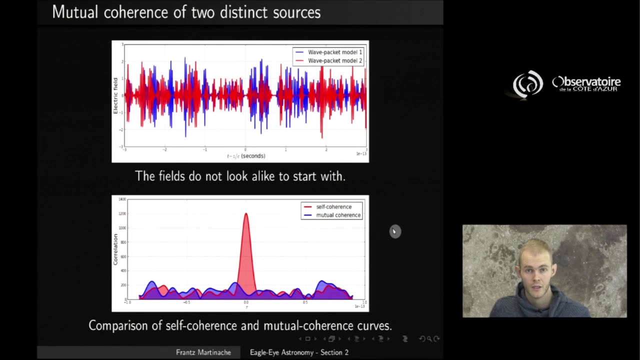 So you can see individual packets popping here and there, And we're very close to the situation where we had two signals that are so delayed in time that they don't look alike at all. If you want to quantify this, we are going to compute the actual self-coherence. 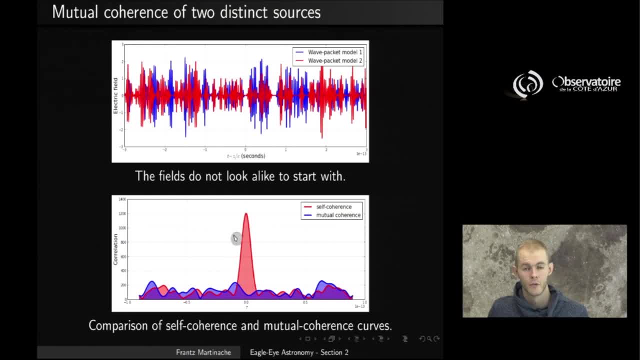 and mutual coherence curves And the red curve that you have here, you may recognize it because it corresponded to the self-coherence function we saw earlier, That is, the coherence between one signal and itself delayed in time. The blue curve, in comparison, corresponds to the mutual coherence function. 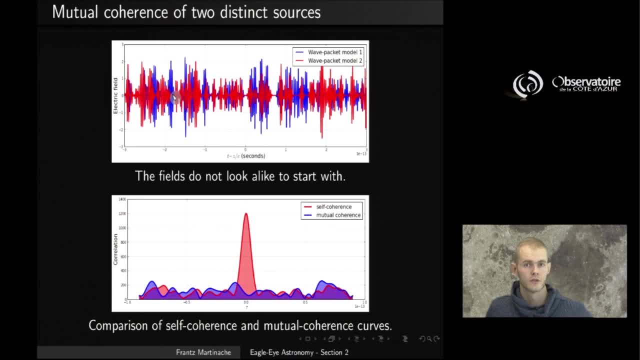 between two different electric fields coming from two different, distinct sources, And you see that that mutual coherence function never gets significantly higher than well. it's very close to zero, And this is keep in mind that this is only by looking at the time scale. 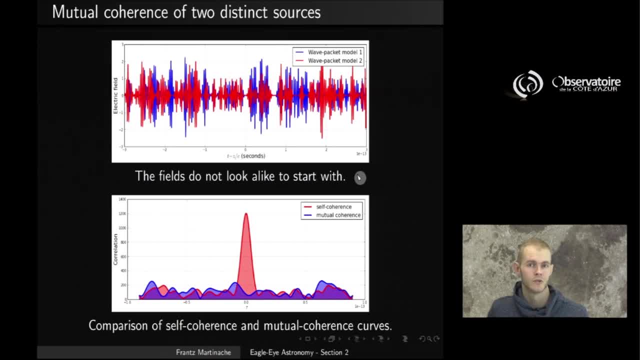 of about 10 to the minus 13 seconds, which is an exposure time so short that we can never actually reach it. Typical exposure times in astronomy are going to be of the order of a second or maybe down to a millisecond, which means that we're not going to average. 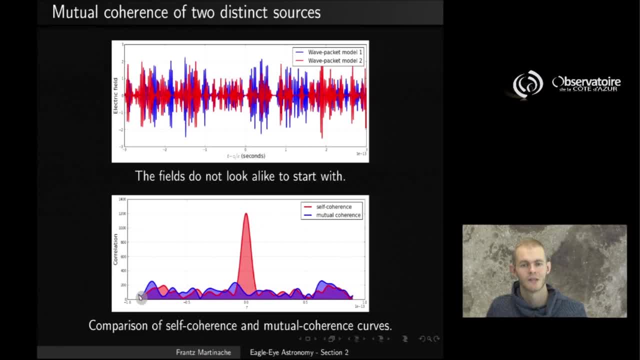 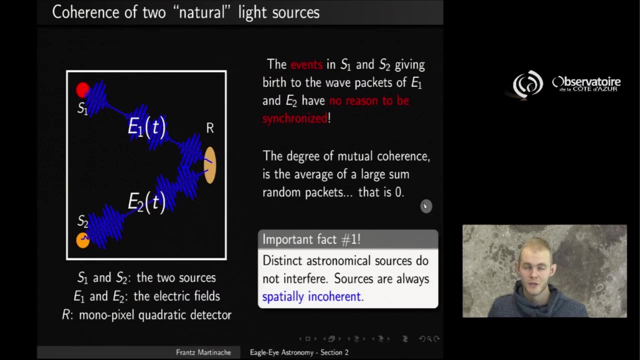 hundreds of events, but actually billions, And so this averaging effect is going to make that the mutual coherence function is essentially zero. So now, if we think about the coherence of two natural light sources, then here we're going to slowly transition toward our application. 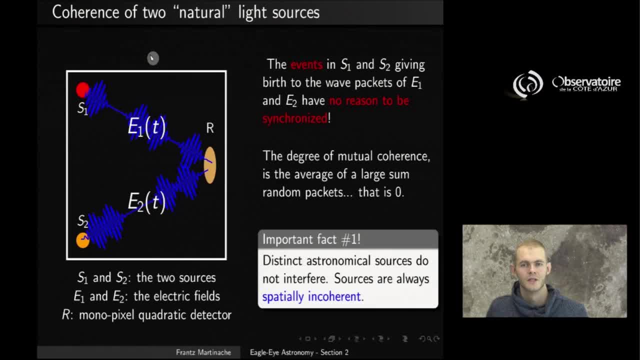 which is actual astronomy. So we can think of two natural light sources as two different stars or two parts of the same star, the left part and the right one, or the top and the bottom or the center of something else, But easiest to think about, 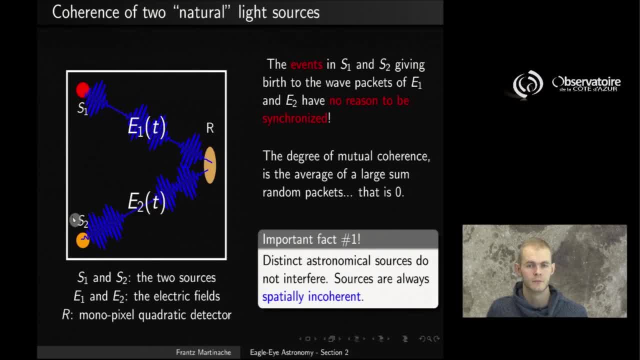 is these two distinct stars, S1 and S2.. Now you realize that the events in S1 and S2 that give birth to the wave packets that make up the bulk of the electric fields, E1 and E2, they have no reason to be synchronized at all. 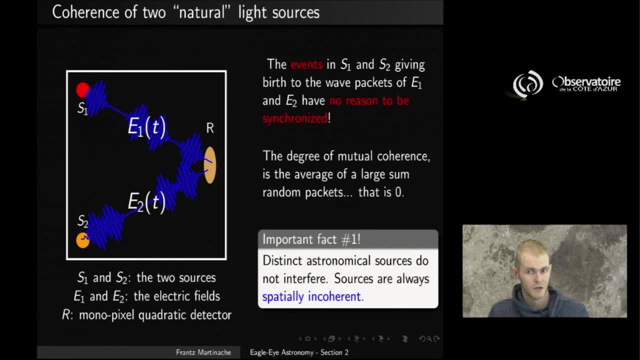 I mean they are different objects or different locations of the same object. The local temperature may be different. There's no reason for the wave packets to be synchronized, And so if we look at one receiver trying to mix the two signals, E1 and E2,, 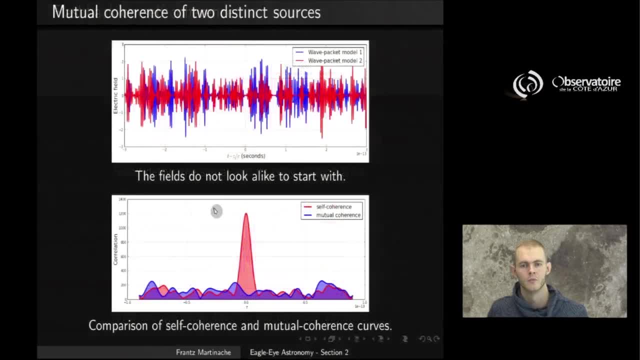 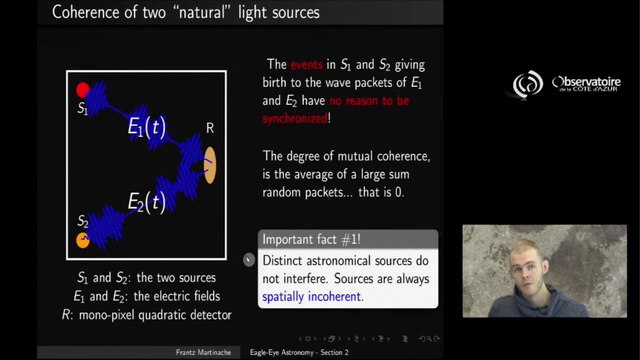 well, just like we saw it in our previous case, here we just have to accept the fact that we are never going to be able to measure any mutual coherence significantly different from zero, And that is a very important fact, One of the most important pieces of information. 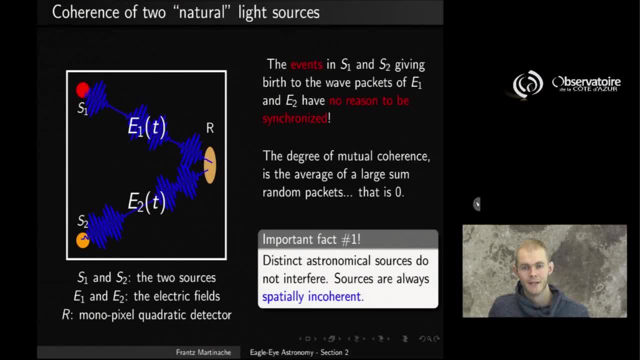 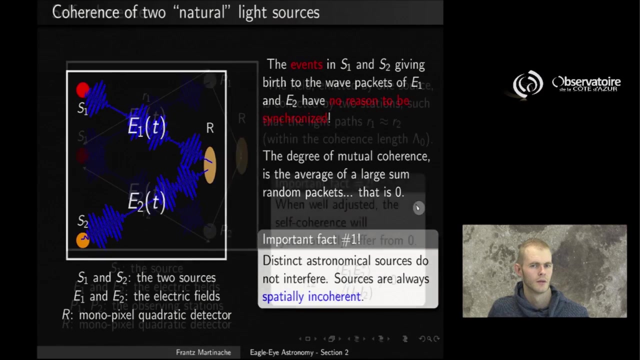 you want to keep in mind in the context of interferometry is that the light of distinct astronomical sources will never interfere with each other. One way to formulate this is to say that sources are going to be spatially incoherent. They are never going to produce interferences. 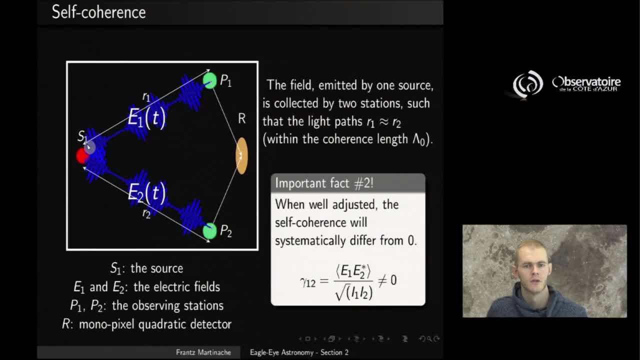 On the other hand, we have self-coherence: If two observing stations look at one object, then the field emitted by that one source is going to reach the stations, And if the distance that links those stations to the source is essentially the same, 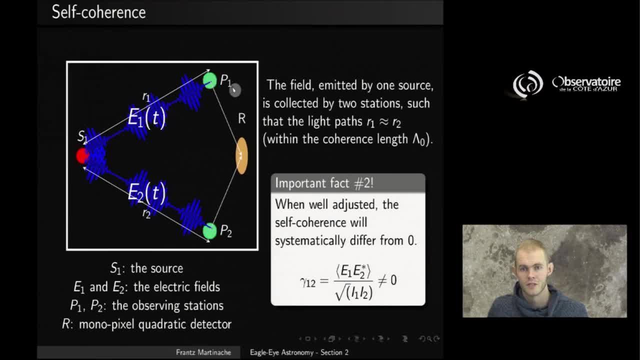 and we've even established a criterion for this. it has to be the same to within this parameter that we've introduced before, called the coherence length, And then, in such circumstances, the wave packets are going to reach the two stations at the same time. 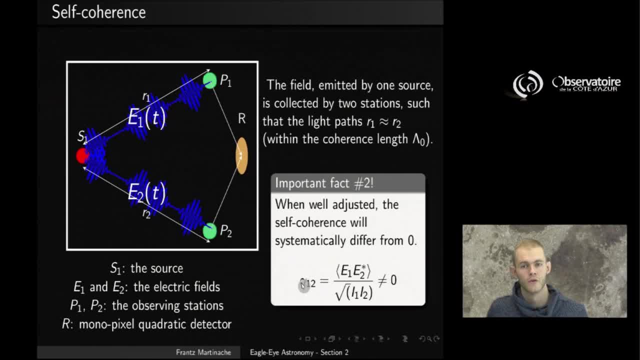 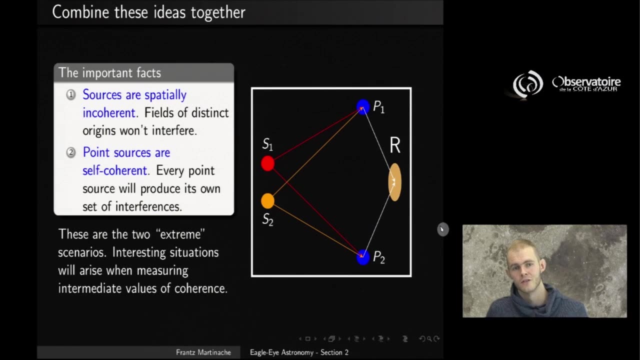 And so if you try and mix them and look for a coherent signal, in this case the coherent signal is going to be always systematically different from zero. If you combine those two ideas together, the two important facts, I repeat, are going to be that: 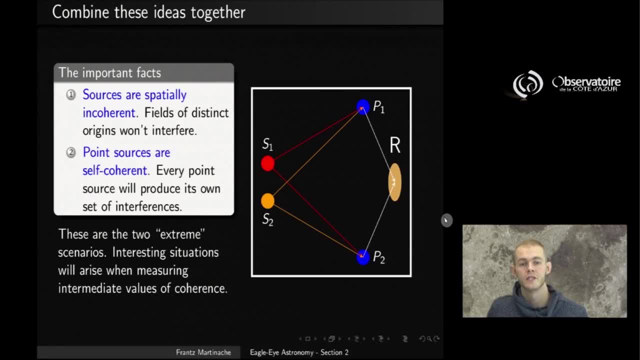 sources are spatially incoherent. The field of distinct origins are never going to interfere with each other. The second fact is that point sources are self-coherent. What that means is that when you perform observations, you're going to observe that every point source is going to produce. 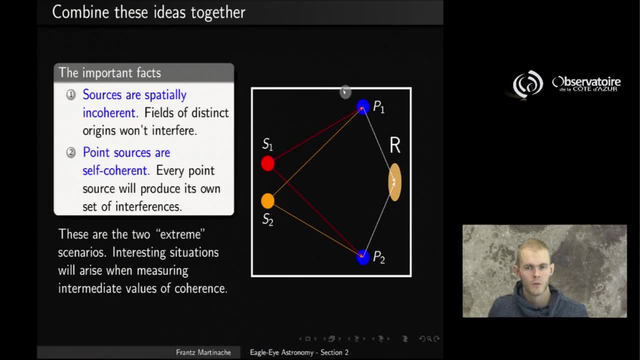 its own set of interferences. We can somehow summarize this situation by this plot here, where we have more than one source, here and also here, simply two that are being observed by two stations simultaneously. The light of the two is never going to interfere. 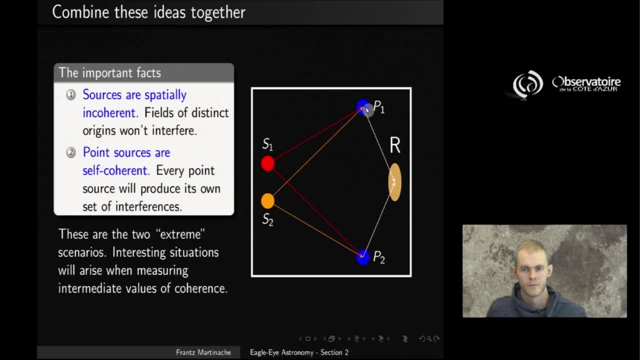 However, the light collected by P1 and P2, the two stations on S1, is going to interfere, And the light collected by the same two stations on S2 is going to interfere. These are really the two extreme scenarios. On the other hand, 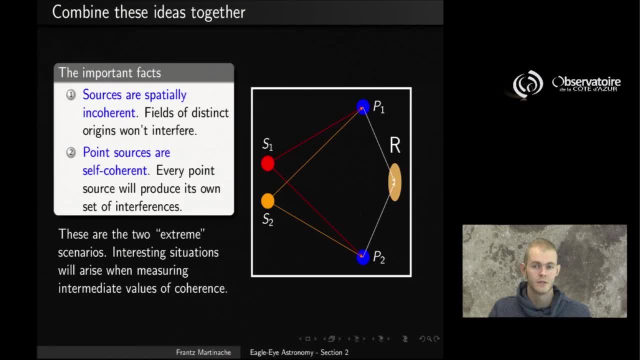 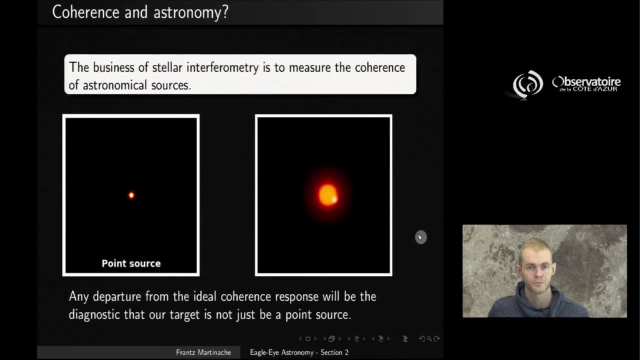 you have zero interference or zero coherence and on the other hand, you have perfect coherence. Of course, the interesting situations will arise when we are measuring intermediate values of coherence, And this is the whole business of stellar interferometry: You want to measure the coherence. 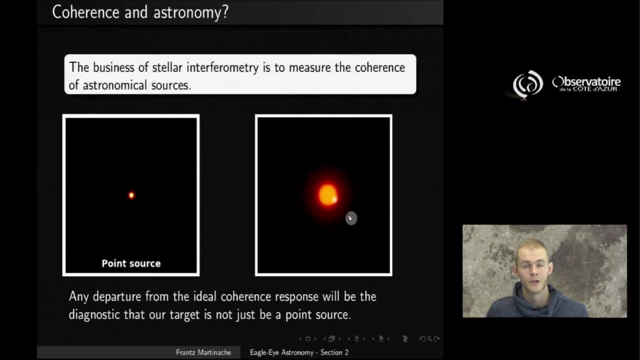 of astronomical sources. We are going to distinguish two types of sources: things that we will refer to as point sources, or perfectly coherent sources, and sources that are different from that, that differ from that, like a resolved object with a companion, for example. 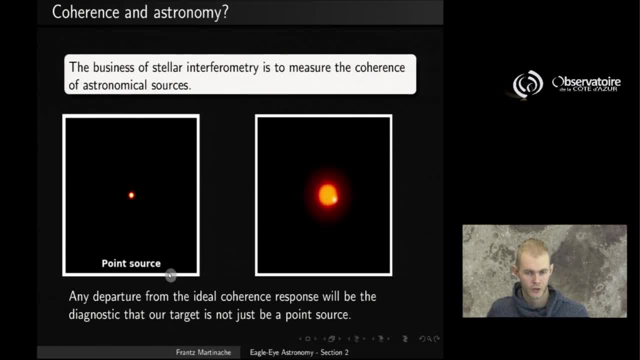 A point source is always going to produce perfect coherence if we manage to make the light reach a detector to within the coherence length, And so any departure from the ideal coherence response we should be getting, according to our theory or the model of our instrument, is going to be a diagnostic that is going to tell us